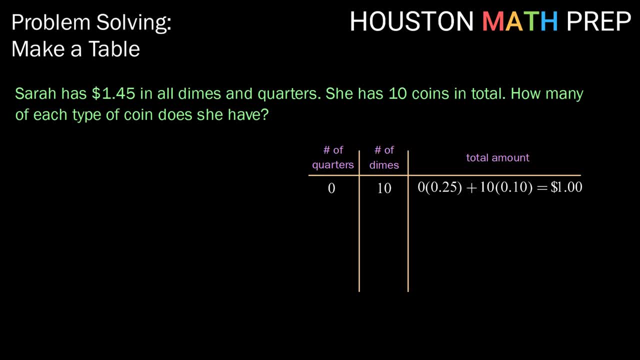 25 cent quarters and 10 10 cent dimes. 10 times 10 cents gives her one dollar. So we know that that combination does not work. Next we could try: what if she has one quarter and nine dimes for her total of 10 coins? Then she would have one 25 cent quarter and nine 10 cent dimes for a. 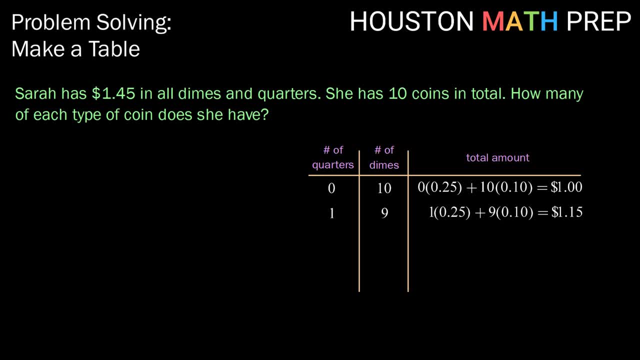 total of $1.15.. Still not the $1.45 that she needs. So if we continue this pattern, we can see that two quarters and eight dimes doesn't quite work. But now we might start to see what we think is a pattern emerging. So when we increased from zero to 10,, 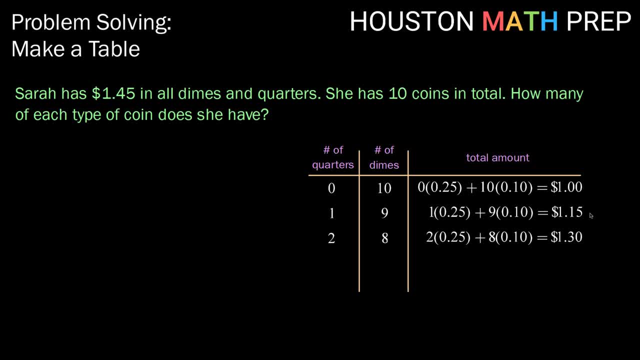 to one quarter, we went from one dollar to one dollar and fifteen cents, And when we went from one quarter to two quarters, we went from one dollar and fifteen cents to one dollar and thirty cents. So so far at least, as we change the number of quarters, 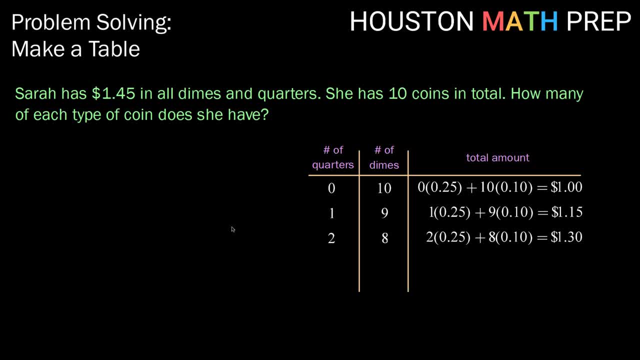 and dimes. we seem to be increasing our total amount by fifteen cents. Let's see if that pattern holds. If so, we should have that three quarters and seven dimes gives us. there it is our total of one dollar and forty-five cents. So Sarah has three quarters and seven. 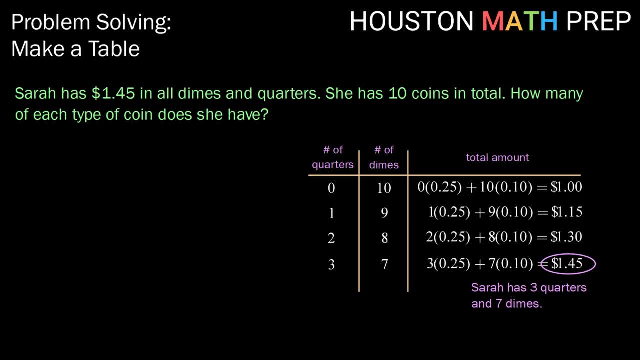 dimes. Okay, so before we end, let's think about looking back. Did we understand the question we were asked- Was making a table here an appropriate strategy? And did we achieve a correct answer? Alright, guys, that does it for this video on problem solving strategy. 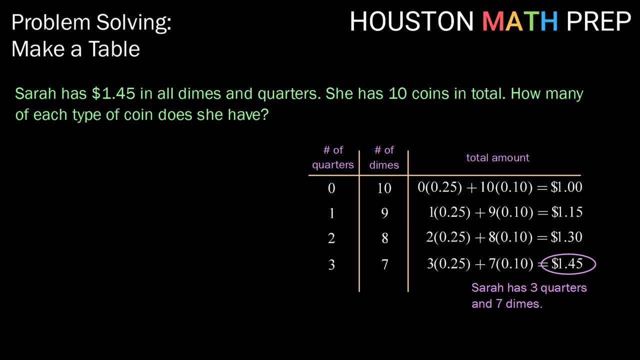 making a table To see more of these. we'll catch you in the next video. 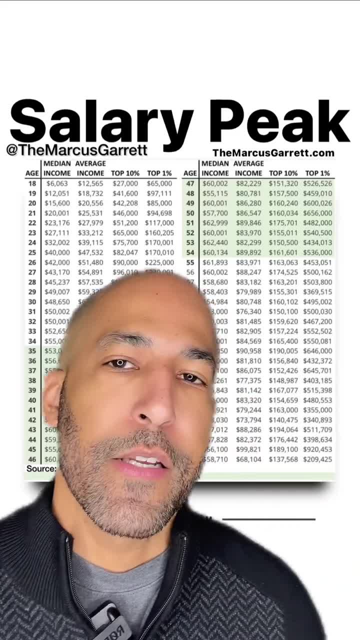 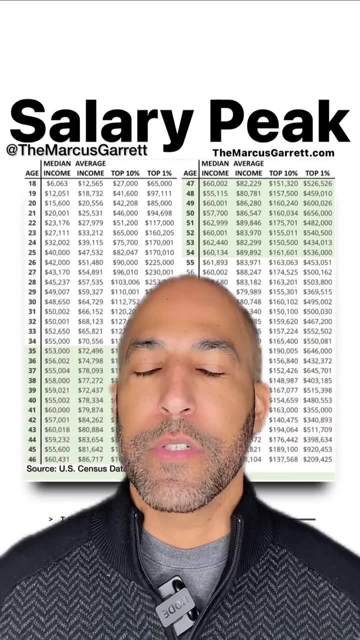 I just posted peak salaries in America on my Instagram, which you can find a link in bio. Peak salaries occur between the ages of 35 and 54, according to the Bureau of Labor Statistics. Then I received a request to add the top 5% of earners.